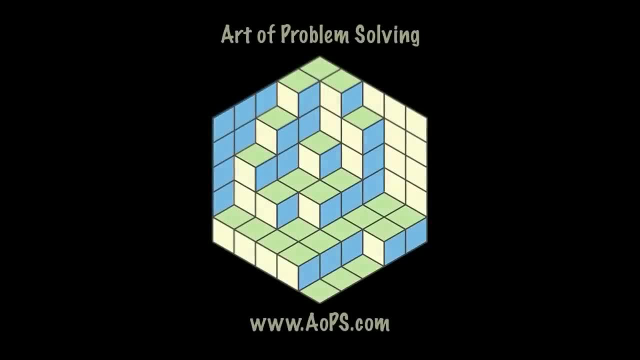 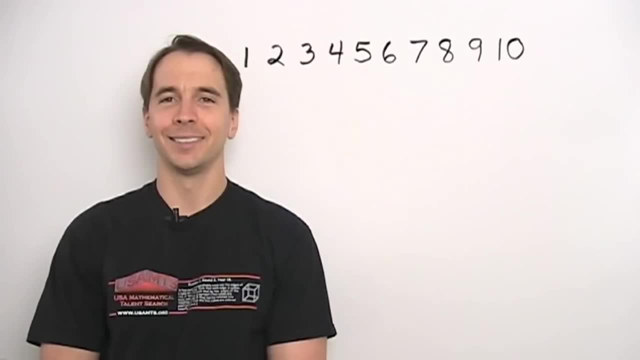 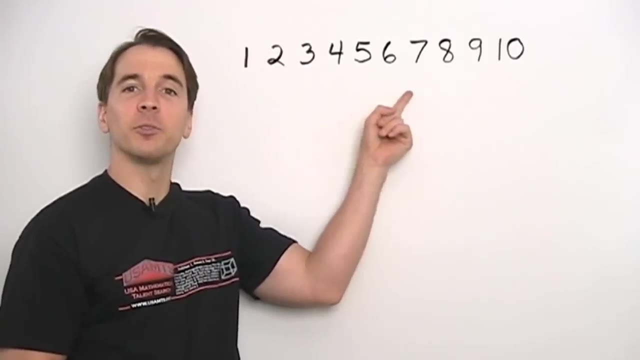 Do you like games? I like games. We're going to play a game. You're going to like this game. I'm going to pick a number from 1 to 10.. I'm going to choose one of these numbers And then you're going to choose a number as well, And if your number 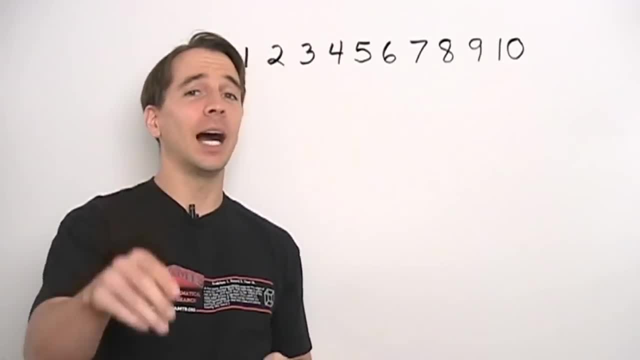 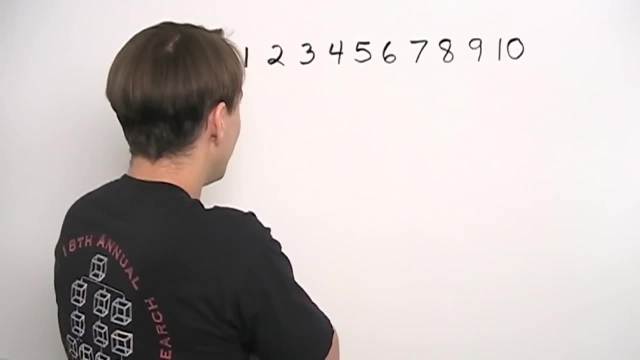 is no more than 2 away from my number. I'm going to send you $1,000.. All right, now I'm going to pick my number. I'm going to look here. I'm going to look at it. I'm looking at my number. Okay, I've got my number. You pick yours. All right, say it out loud. 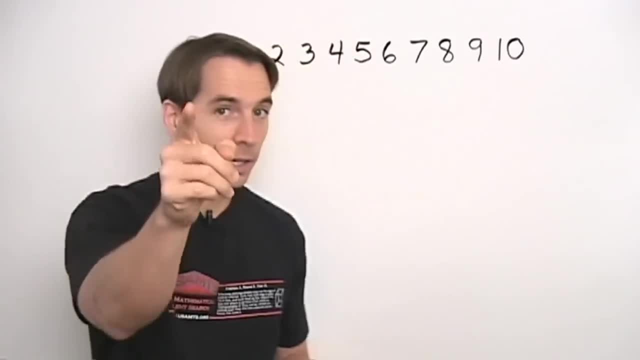 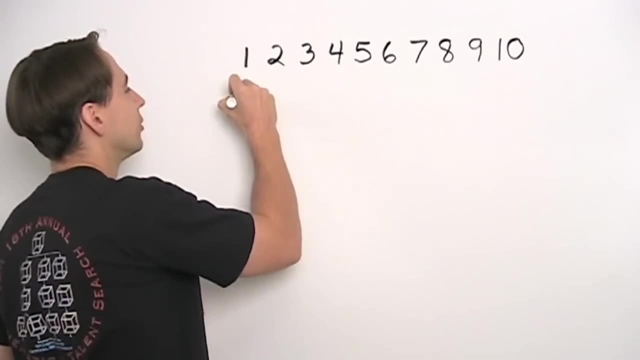 Say it out loud, I want to hear it, so you don't change it later. Okay, I got your number. Now we're going to find the probability that you win. So that's what we're going to compute here: probability that you win. 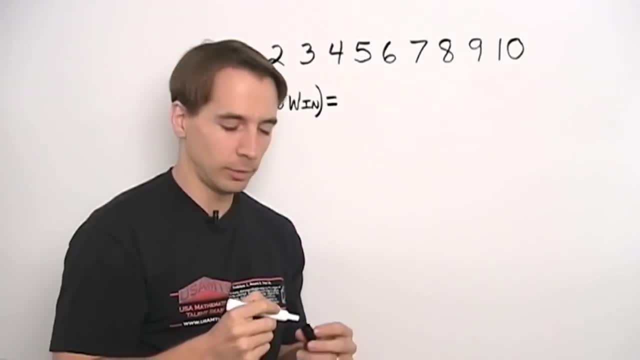 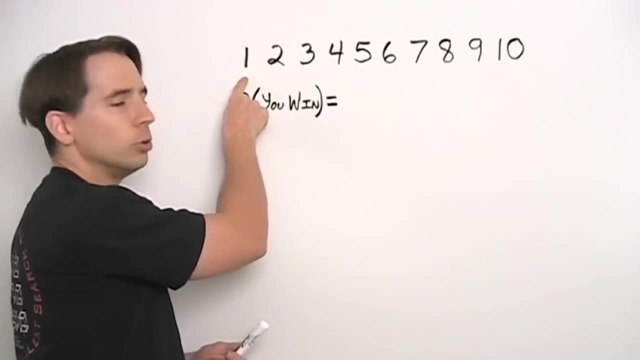 And first we're going to do a little strategy here. You have to be within 2 of my number, So would you pick 1?? If you pick 1, you only win if I pick 1,, 2, or 3.. However, if you picked 5,, 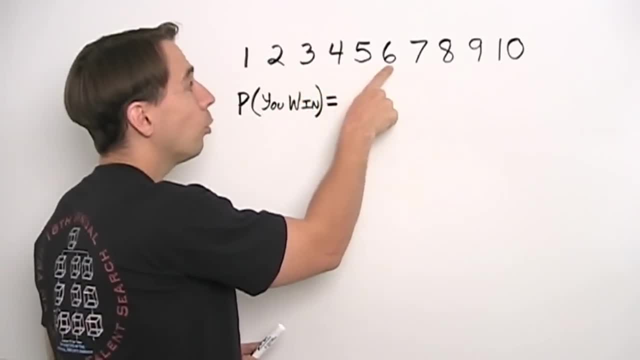 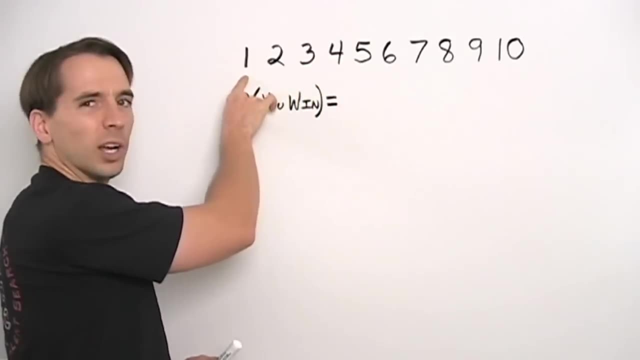 you'd win if I'm 2 below at 3 or 4, or above 6 or 7.. So you have 5 numbers that I could have and you'd still win if you'd pick 5.. So you're not going to pick 1, because that only gives you. 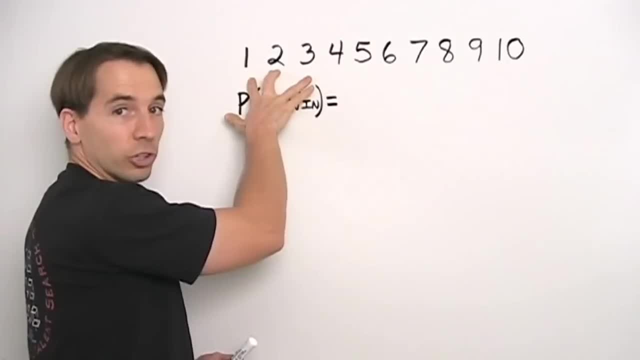 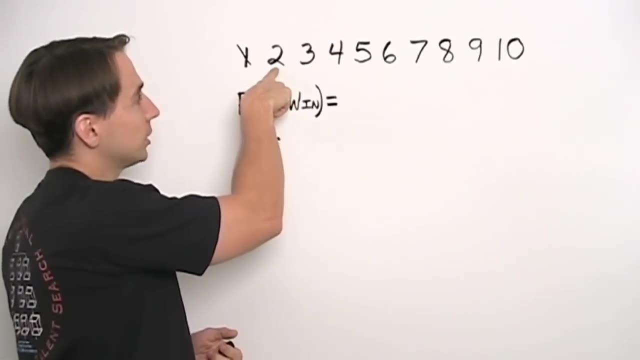 3 chances to win and you can pick 3. And get all 3 of those chances covered and still get 2 others. So you're not going to pick 1.. And for pretty much the same reason, you're not going to pick 2, because if you pick 2, you only cover 1,, 2,, 3, and 4.. 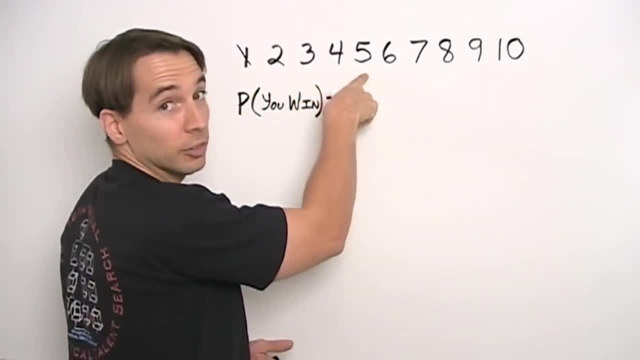 But you could pick 3 instead and cover 1,, 2,, 3, and 4, and cover 5 as well. So you're not going to pick 2 either. You're not going to pick 9.. You're not going to pick 10.. You're going to pick one of these numbers in the middle. 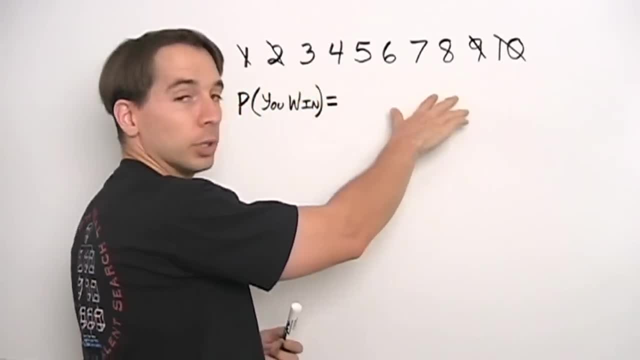 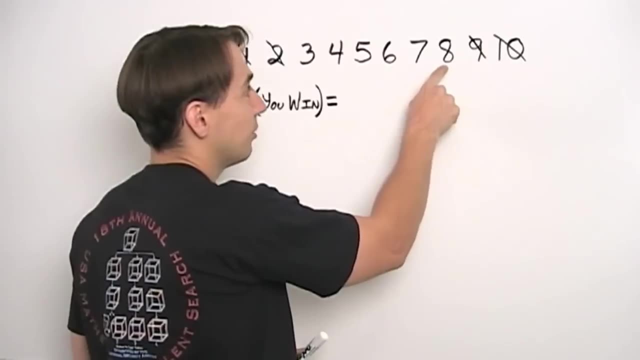 And when you pick one of these numbers in the middle, no matter what number you pick, you'll have 5 chances to win. For example, if you picked 7, you're going to win If I pick 5,, 6,, 7,, 8, or 9.. 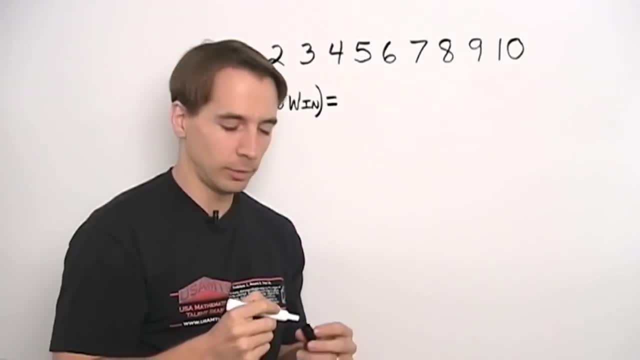 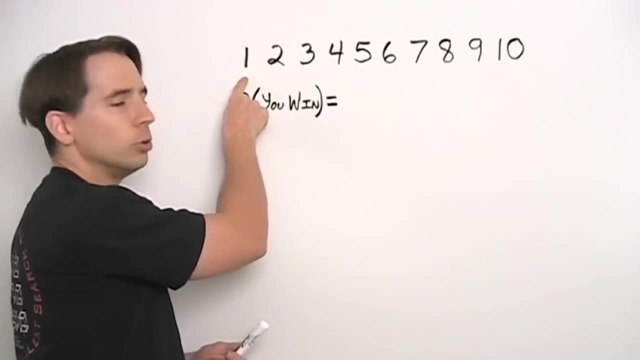 And first we're going to do a little strategy here. You have to be within 2 of my number, So would you pick 1?? If you pick 1, you only win if I pick 1,, 2, or 3.. However, if you picked 5,, 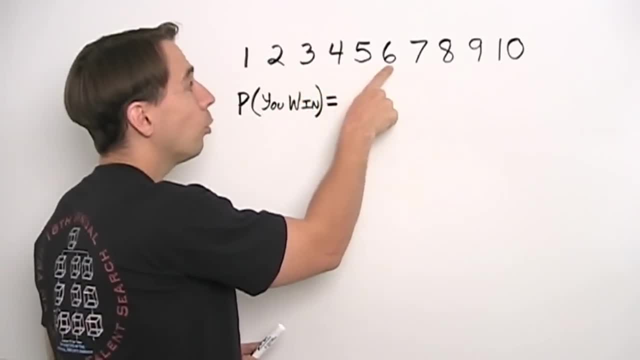 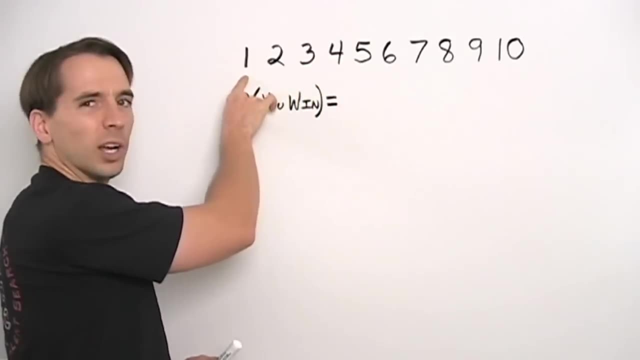 you'd win if I'm 2 below at 3 or 4, or above 6 or 7.. So you have 5 numbers that I could have and you'd still win if you'd pick 5.. So you're not going to pick 1, because that only gives you. 3 chances to win and you can pick 3. And get all 3 of those chances covered and still get 2 others. So you're not going to pick 1.. And for pretty much the same reason, you're not going to pick 2, because if you pick 2, you only cover 1,, 2,, 3, and 4.. 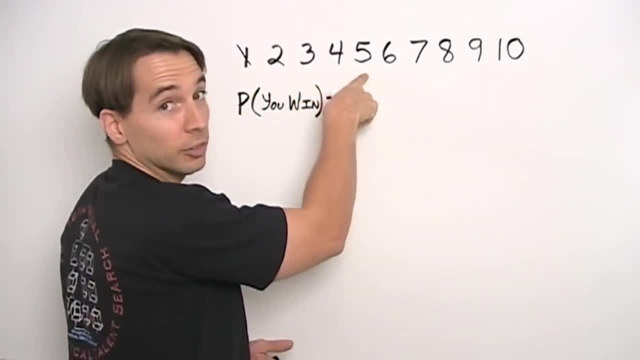 But you could pick 3 instead and cover 1,, 2,, 3, and 4, and cover 5 as well. So you're not going to pick 2 either. You're not going to pick 9.. You're not going to pick 10.. You're going to pick one of these numbers in the middle. 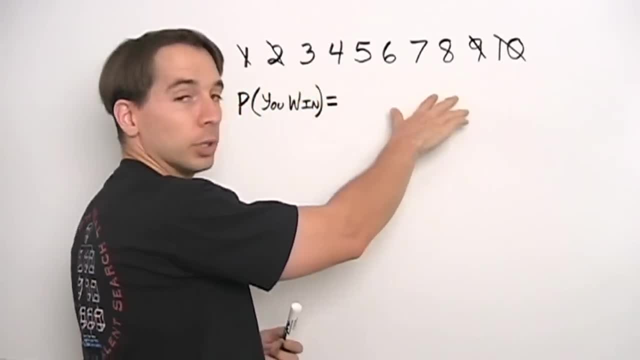 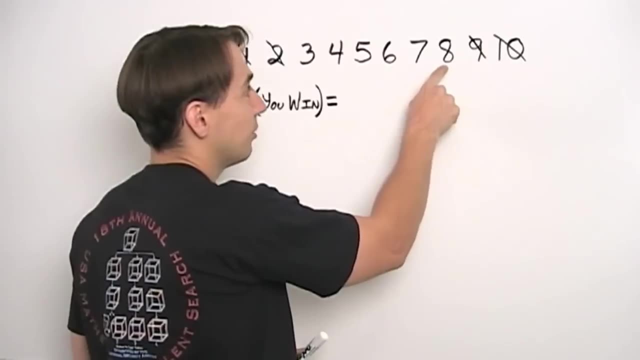 And when you pick one of these numbers in the middle, no matter what number you pick, you'll have 5 chances to win. For example, if you picked 7, you're going to win If I pick 5,, 6,, 7,, 8, or 9.. 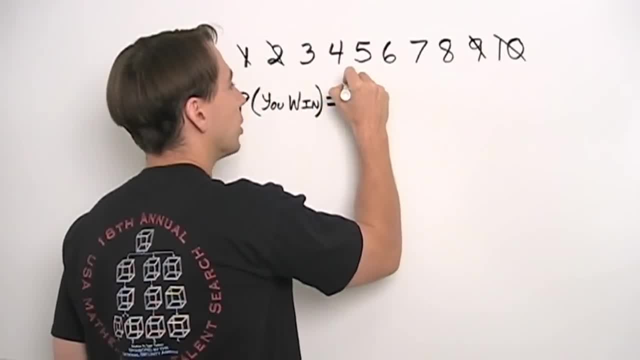 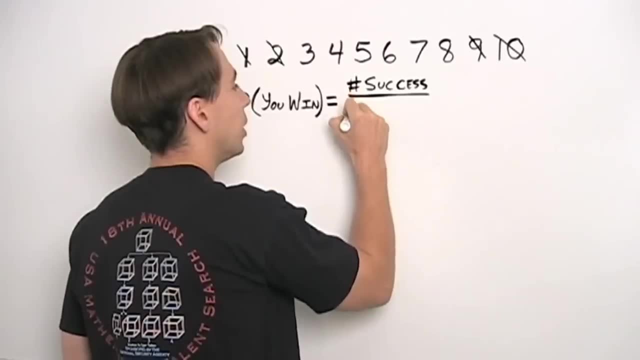 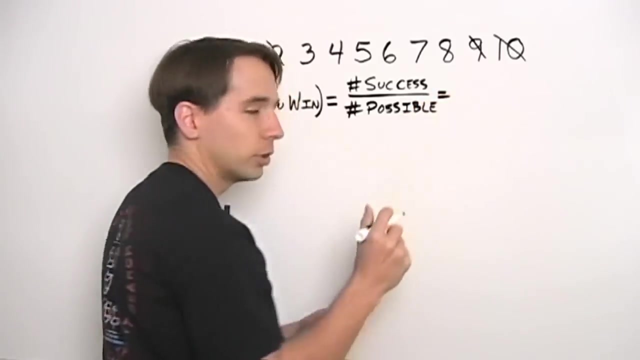 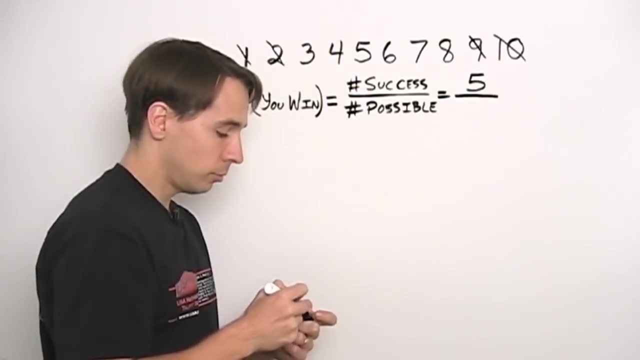 So, the probability you win? well, we're going to do this the normal way. We're going to count the number of successes over the number of possible. And we've just seen that, if you follow your best strategy, which I'm sure you did, you have 5 ways to win. 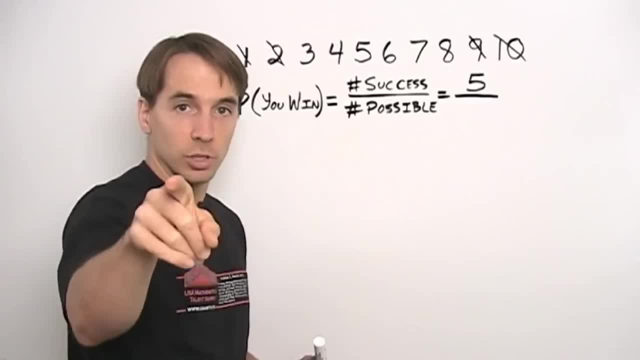 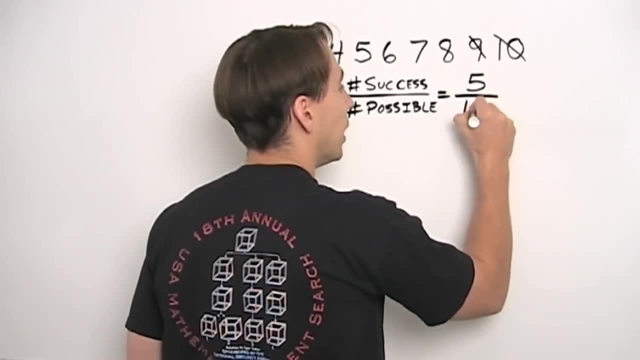 Whichever of these numbers you choose, There are 5 numbers that I can choose and you're going to win $1,000.. Now the number of possible. I can pick any of these, 10.. So the number of possible is 10.. 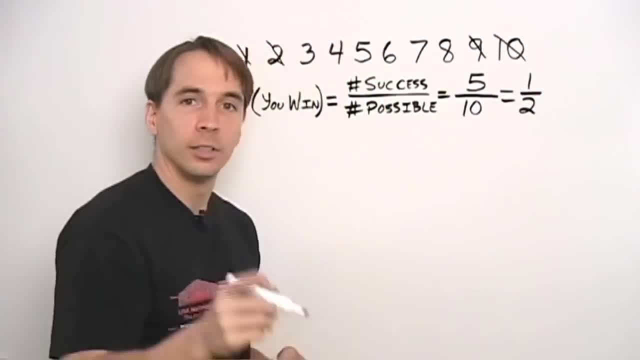 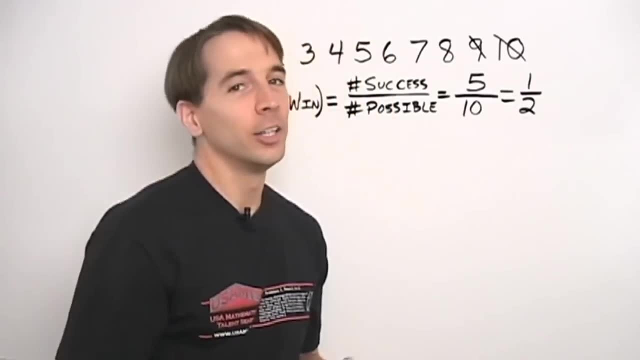 So the probability is 1 half that you're going to win $1,000.. Now, what was your number? Yeah, yeah, I remember that You missed by 4.. I'm sorry So you don't win, but that was a nice try. 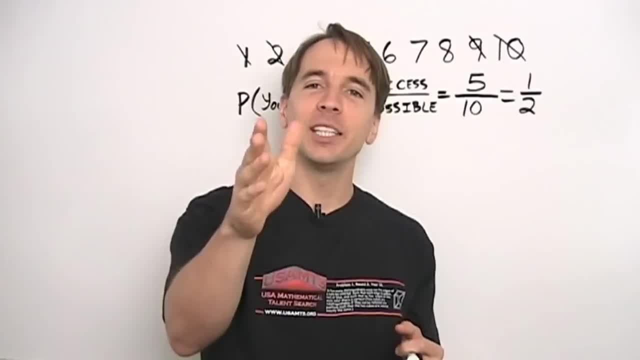 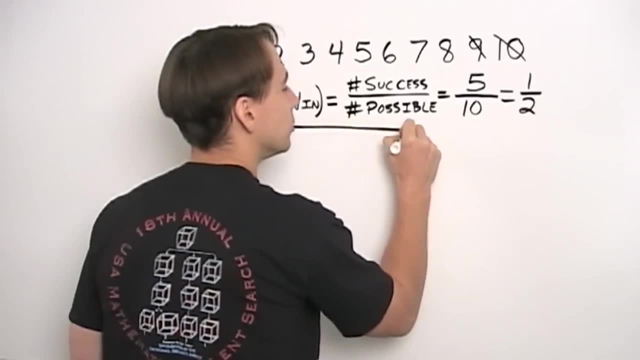 But you see, I'm a nice guy, So I'm going to give you another chance. We're going to change the game a little bit. We're going to change the game a little bit. Instead of picking one of these whole numbers, I'm going to pick any real number, from 1 to 10.. 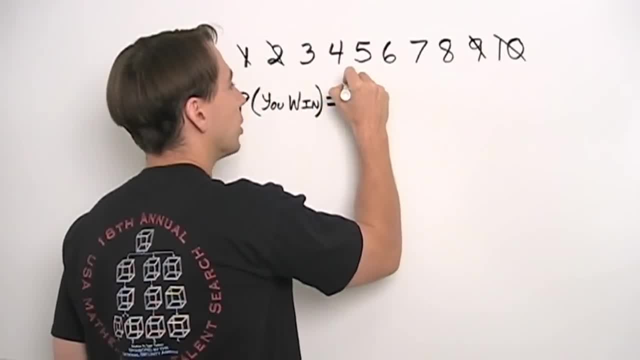 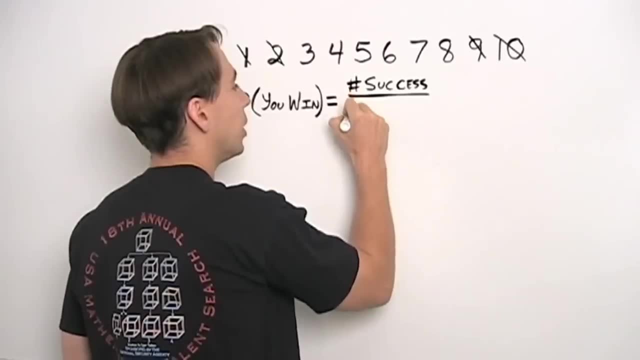 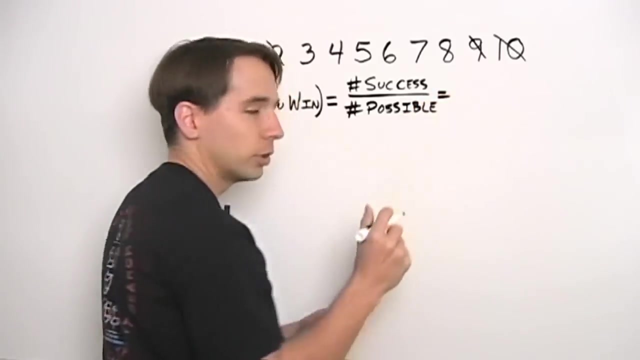 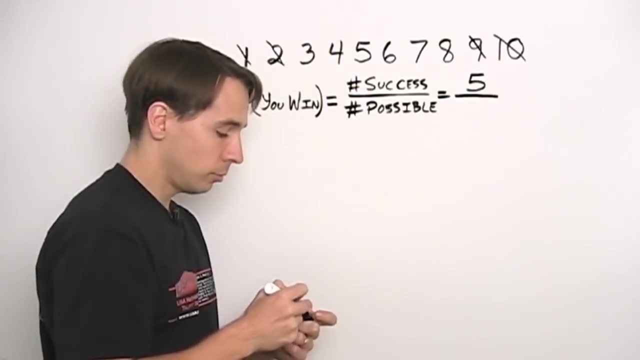 So, the probability you win? well, we're going to do this the normal way. We're going to count the number of successes over the number of possible. And we've just seen that, if you follow your best strategy, which I'm sure you did, you have 5 ways to win. 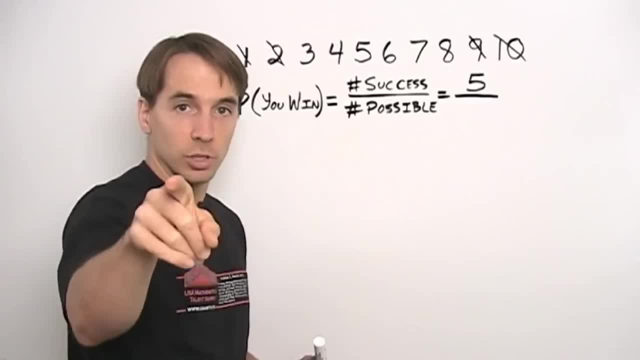 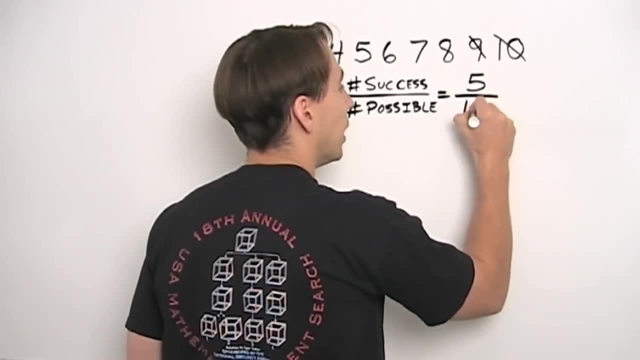 Whichever of these numbers you choose, There are 5 numbers that I can choose and you're going to win $1,000.. Now the number of possible. I can pick any of these, 10.. So the number of possible is 10.. 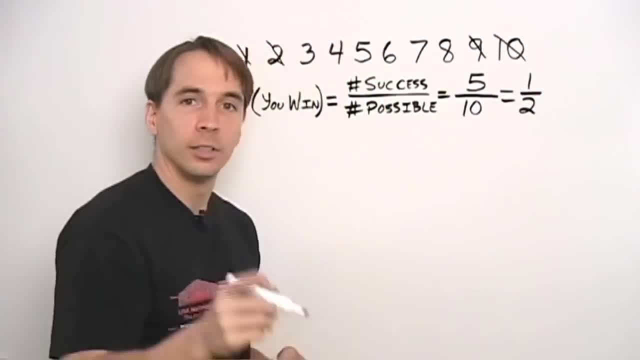 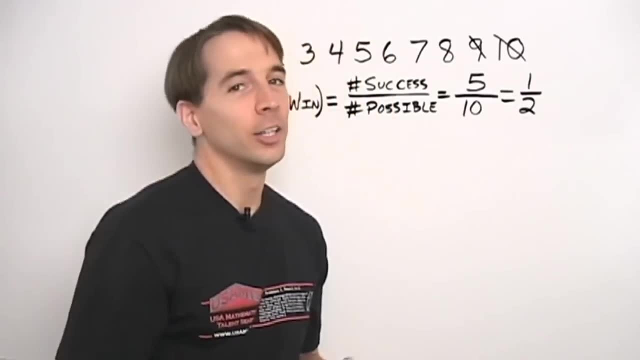 So the probability is 1 half that you're going to win $1,000.. Now, what was your number? Yeah, yeah, I remember that You missed by 4.. I'm sorry So you don't win, but that was a nice try. 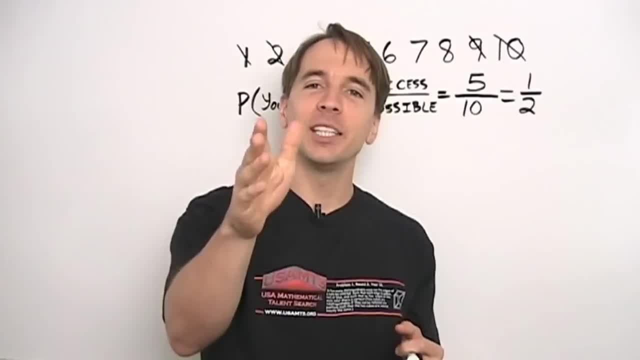 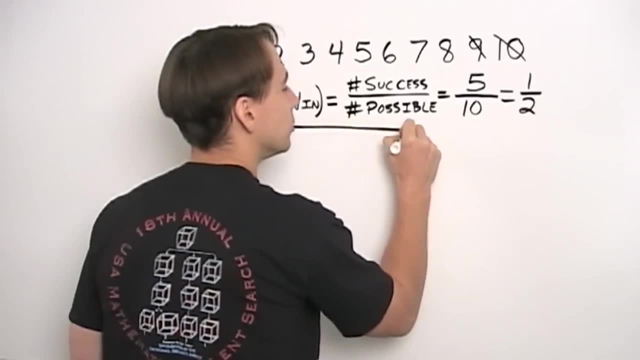 But you see, I'm a nice guy, So I'm going to give you another chance. We're going to change the game a little bit. We're going to change the game a little bit. Instead of picking one of these whole numbers, I'm going to pick any real number, from 1 to 10.. 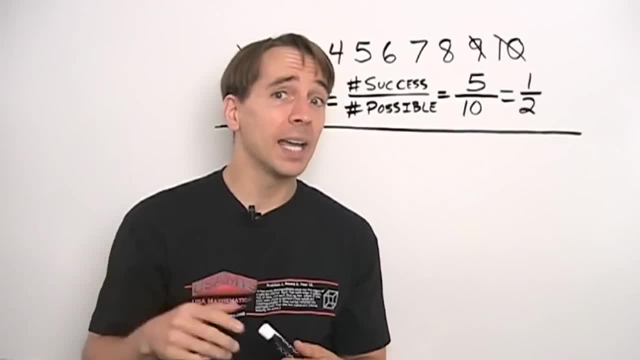 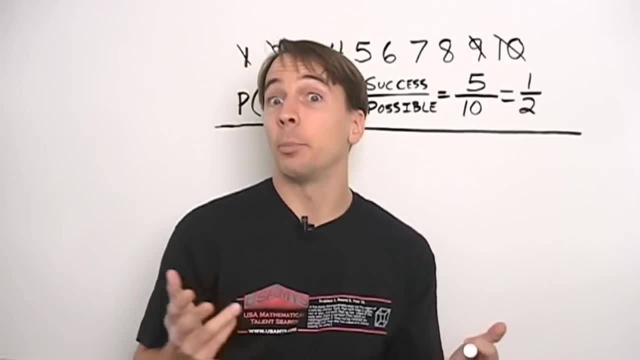 I could pick the square root of 17.. I could pick pi. I could pick 6 and a third, And you can do the same. All right, You know, you can pick pi plus 2,, pi plus 7.. No, you can't pick pi plus 7, because that's more than 10.. 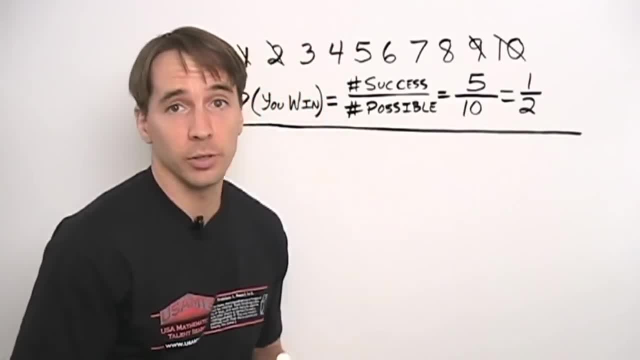 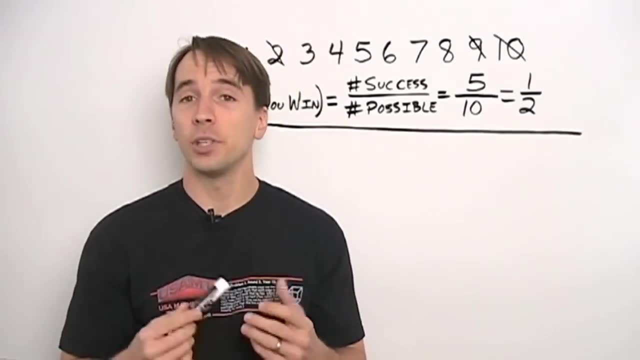 But you could pick the square root of 3.. You could pick 3 times the square root of 3.. And once again, we're going to do the same thing as before: if you're within 2.. If you're within 2 of my number, then you're going to win $1,000.. 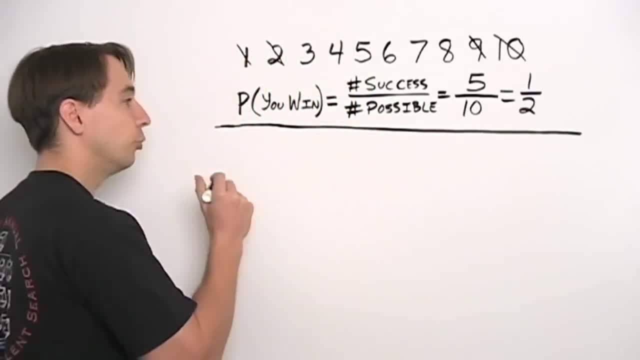 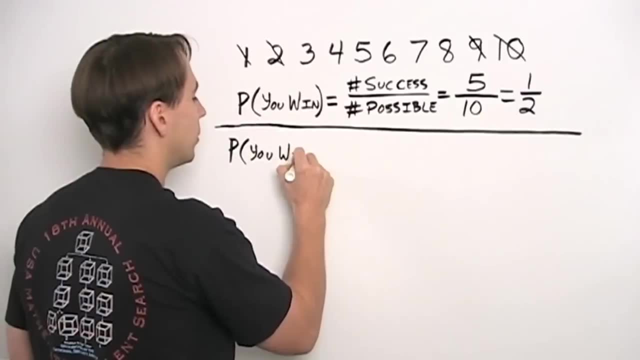 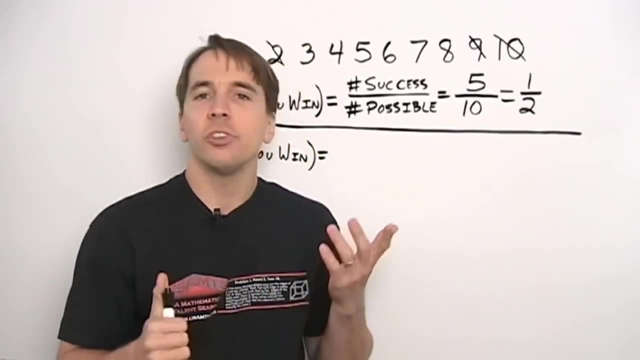 So, once again, we're going to find the probability that you win, Probability that you win, And we'll start off. let's see if we did the number of successes over the number of possible outcomes. well, let's see how many possible outcomes are there, if I can pick any number from 1 to 10?. 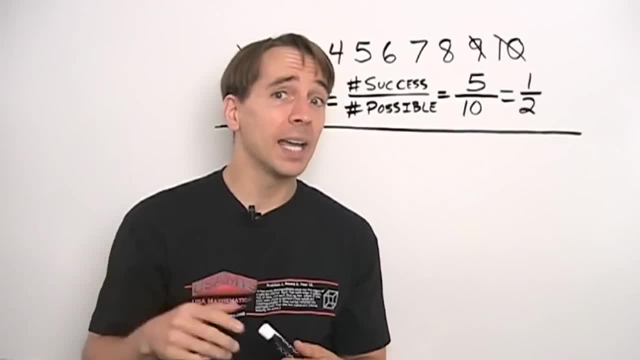 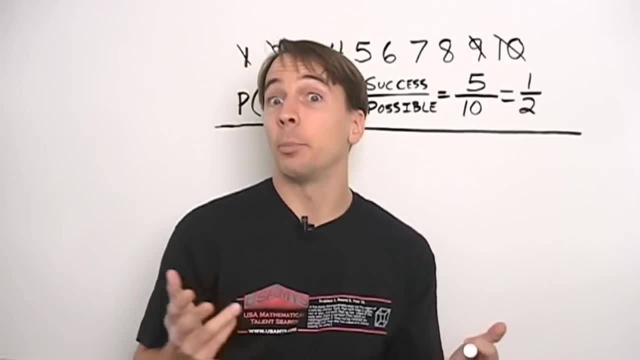 I could pick the square root of 17.. I could pick pi. I could pick 6 and a third, And you can do the same. All right, You know, you can pick pi plus 2,, pi plus 7.. No, you can't pick pi plus 7, because that's more than 10.. 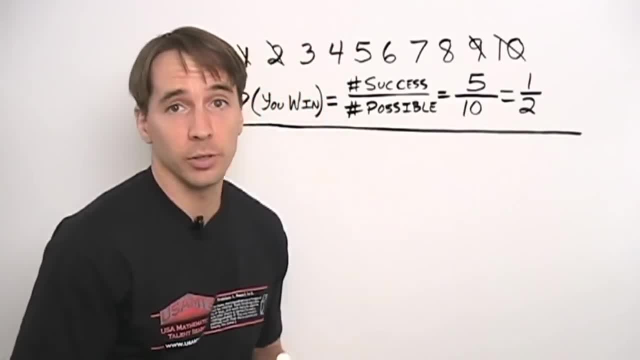 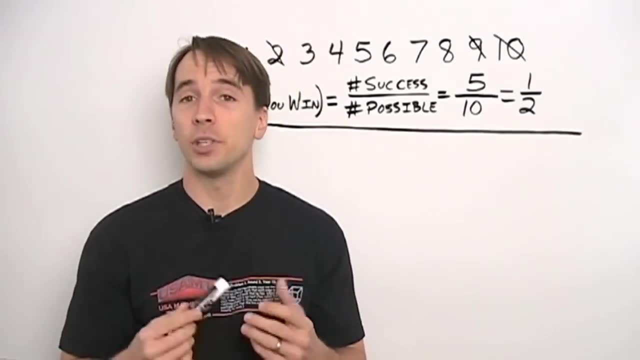 But you could pick the square root of 3.. You could pick 3 times the square root of 3.. And once again, we're going to do the same thing as before: if you're within 2.. If you're within 2 of my number, then you're going to win $1,000.. 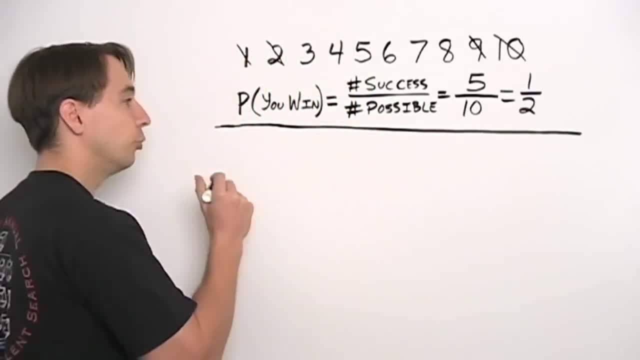 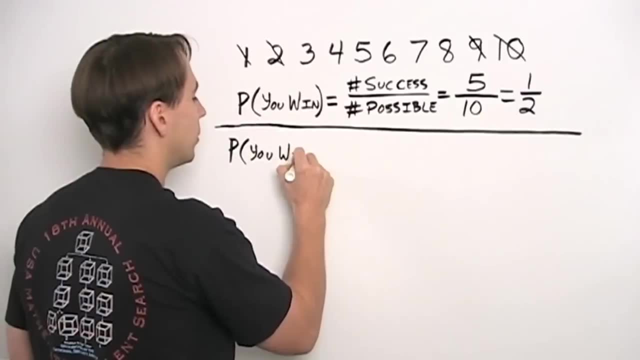 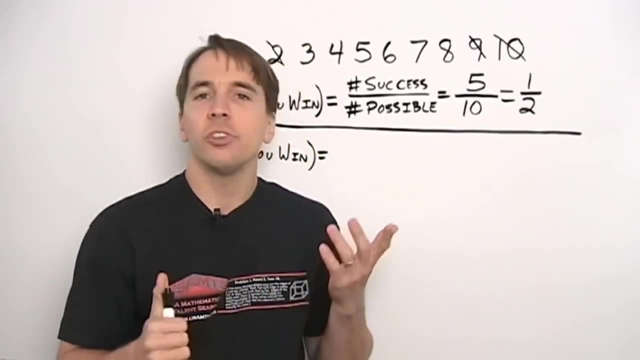 So, once again, we're going to find the probability that you win, Probability that you win, And we'll start off. let's see if we did the number of successes over the number of possible outcomes. well, let's see how many possible outcomes are there, if I can pick any number from 1 to 10?. 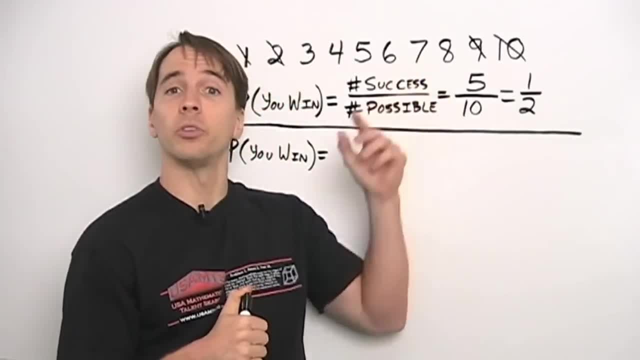 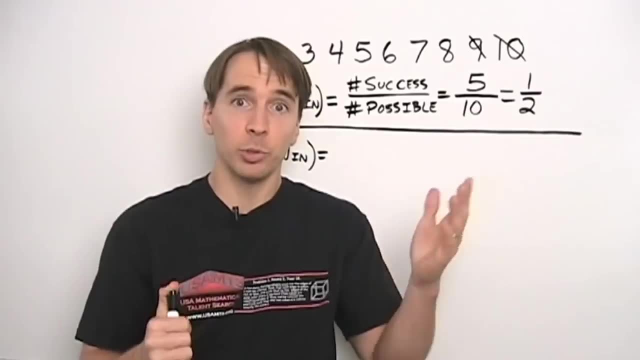 That's a problem, right? Because I'm not just doing whole numbers anymore, I'm doing all real numbers And we can't count those from 1 to 10.. You can't just line up those real numbers and go 1,, 2,, 3,, 4.. 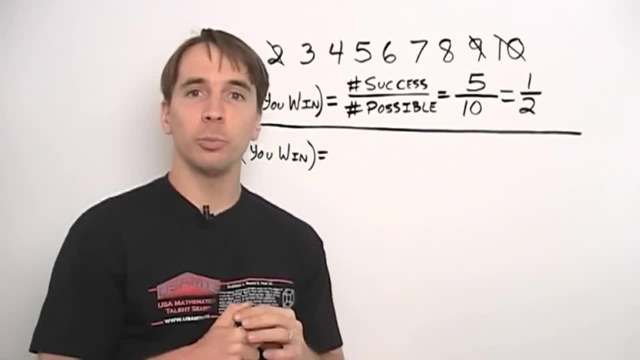 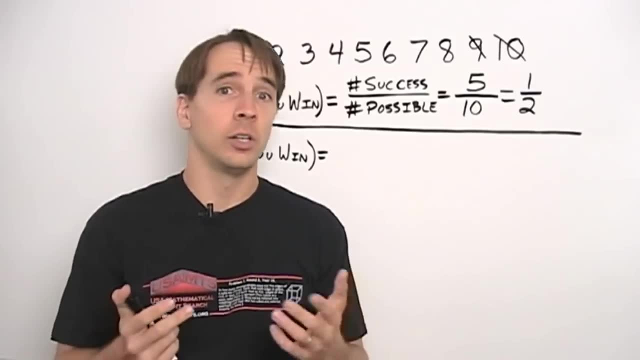 That's a problem. Our number of possibilities is infinite And our number of successes you know. if you picked 7 and a half, well, you win. if I'm anywhere from 5 and a half to 9 and a half. 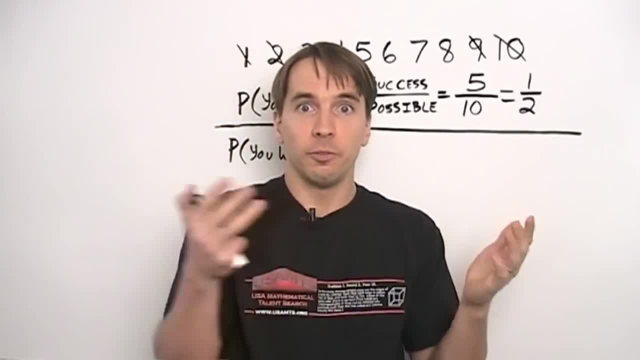 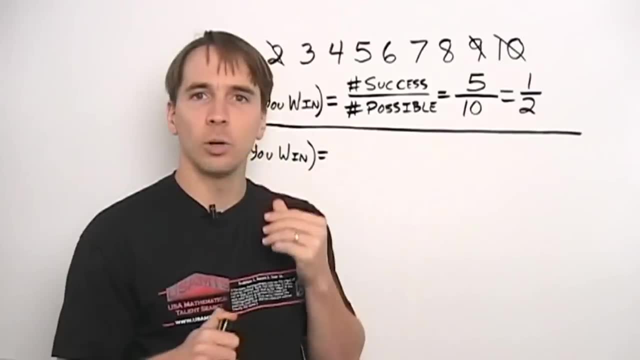 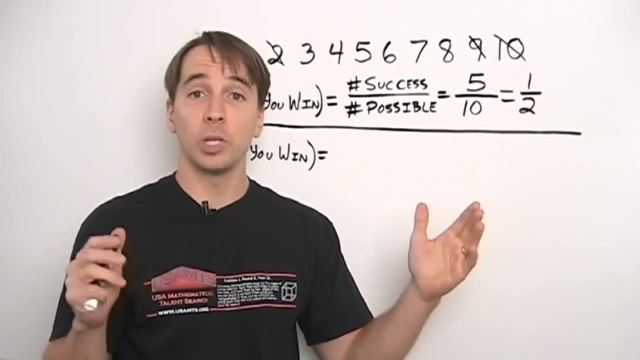 But there are infinitely many real numbers, from 5 and a half to 9 and a half. So this number of successes over a number of possible, that's not going to work. We need to think of some way to deal with this, And the problem here is our possible choices are what we call continuous. 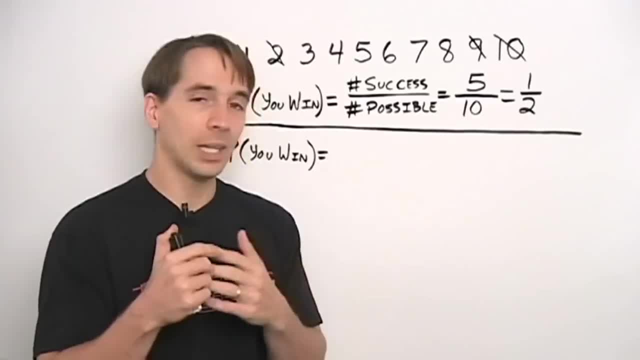 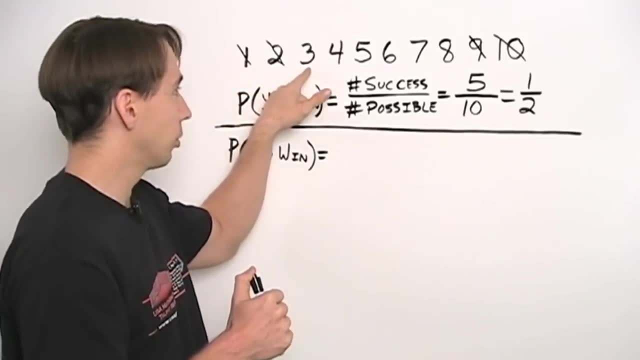 You know any two numbers, well, you can find a number between them. We can't just line them up and count them. And we can line them up and count them like this: We say that's discrete, We can count them 1,, 2,, 3,, 4.. 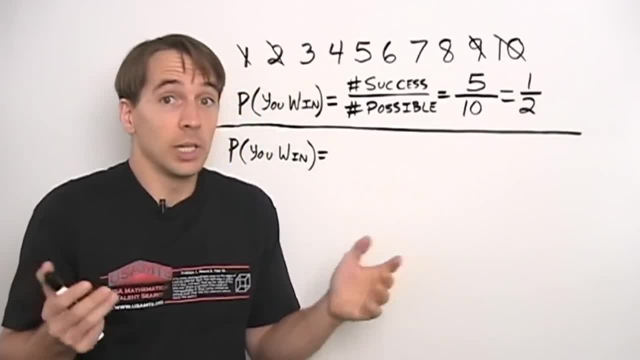 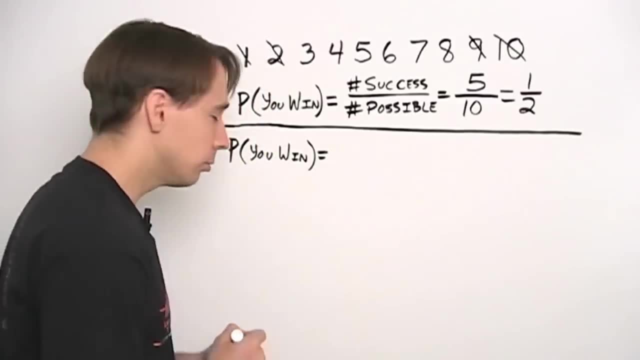 But when we're choosing from any real number- from 1 to 10, it's not discrete anymore. We can't count them, So what can we do with them? Well, we can draw a picture of them And we can use a number line. 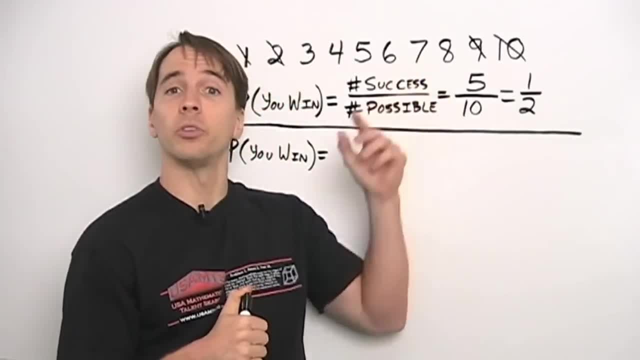 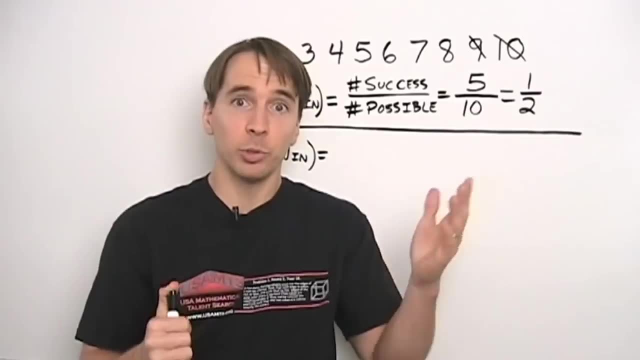 That's a problem, right? Because I'm not just doing whole numbers anymore, I'm doing all real numbers And we can't count those from 1 to 10.. You can't just line up those real numbers and go 1,, 2,, 3,, 4.. 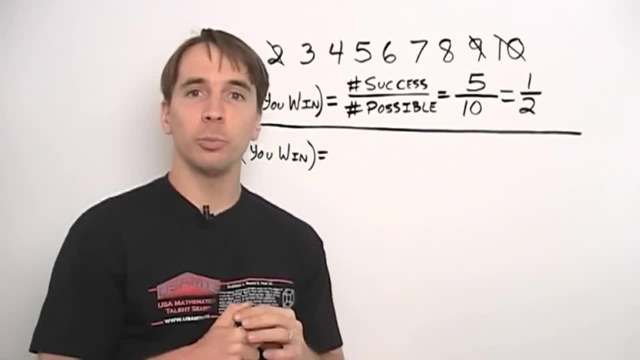 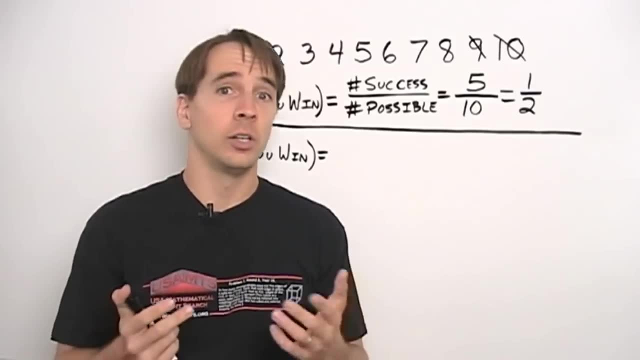 That's a problem. Our number of possibilities is infinite And our number of successes you know. if you picked 7 and a half, well, you win. if I'm anywhere from 5 and a half to 9 and a half. 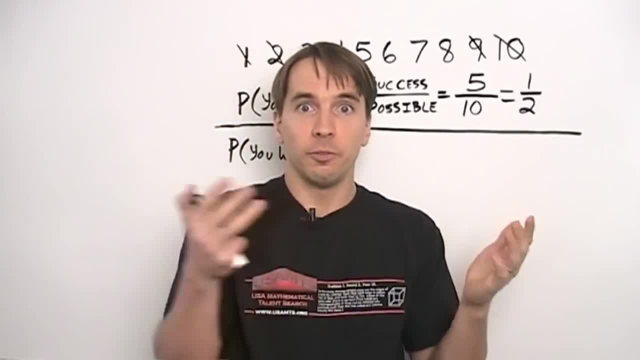 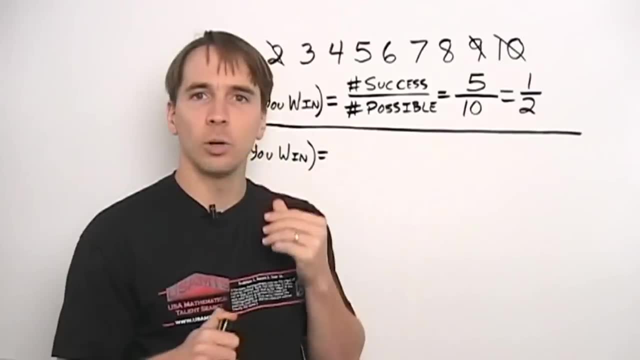 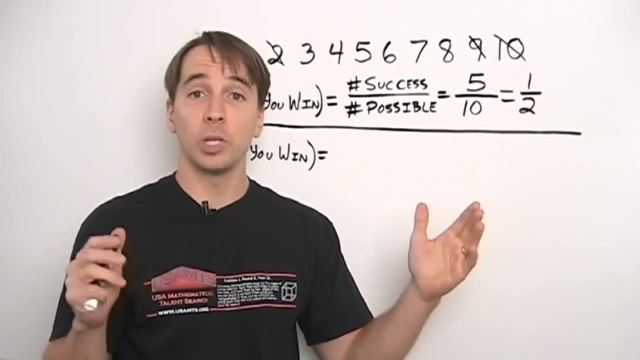 But there are infinitely many real numbers, from 5 and a half to 9 and a half. So this number of successes over a number of possible, that's not going to work. We need to think of some way to deal with this, And the problem here is our possible choices are what we call continuous. 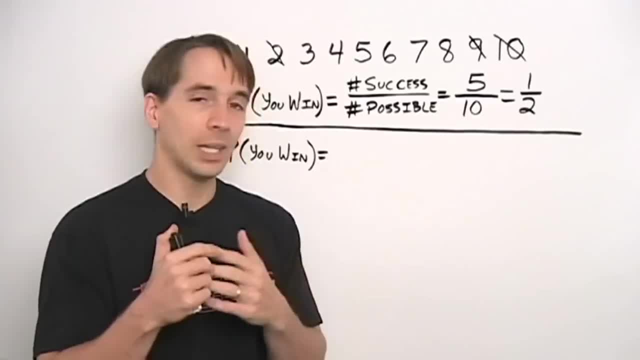 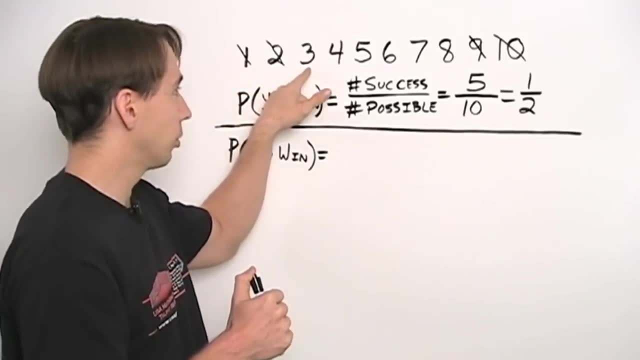 You know any two numbers, well, you can find a number between them. We can't just line them up and count them. And we can line them up and count them like this: We say that's discrete, We can count them 1,, 2,, 3,, 4.. 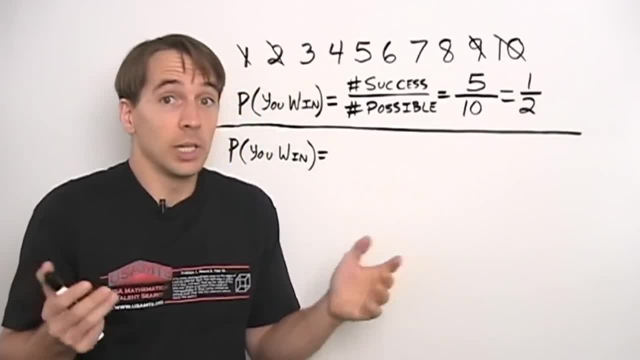 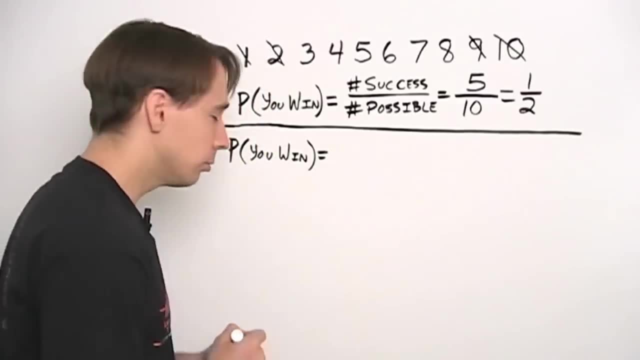 But when we're choosing from any real number- from 1 to 10, it's not discrete anymore. We can't count them, So what can we do with them? Well, we can draw a picture of them And we can use a number line. 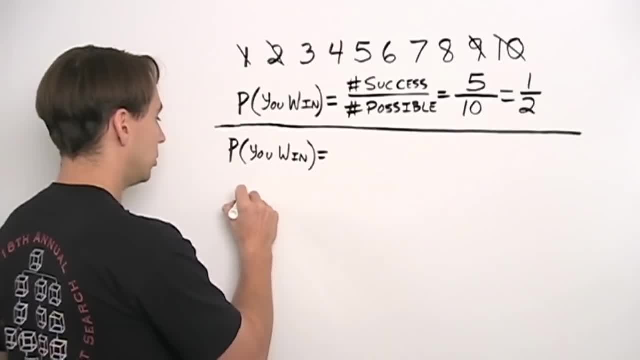 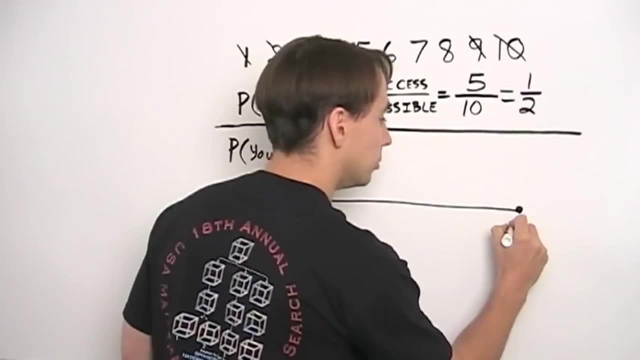 Let's go ahead and look at that. We'll go ahead and draw a number line. Here's our number line And our number line goes from 1 to 10.. Because I can choose any number on the number line from 1 to 10.. 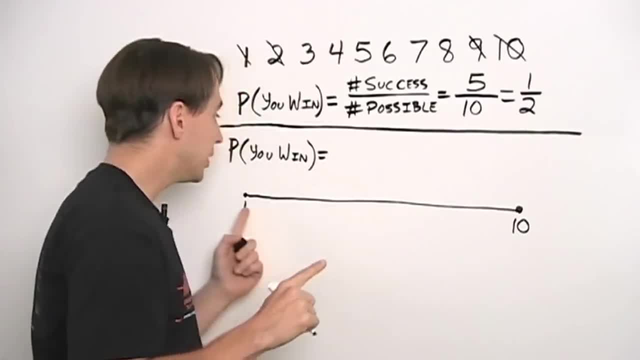 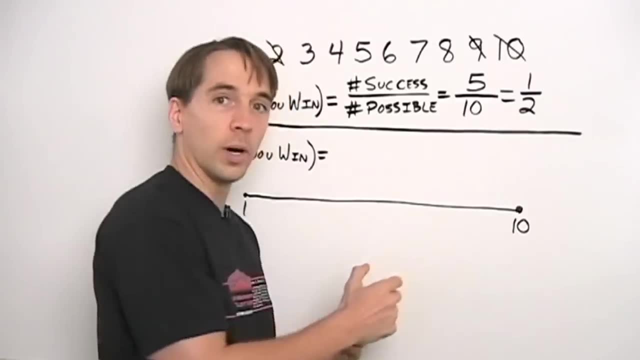 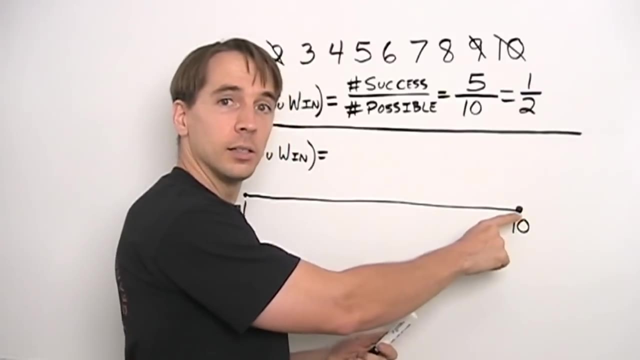 And aha, now we see a way to measure our possible region. There are tools to measure these continuous quantities. Geometry has them, And one of those tools is length. I can pick any number from 1 to 10.. And the length of this region is 9.. 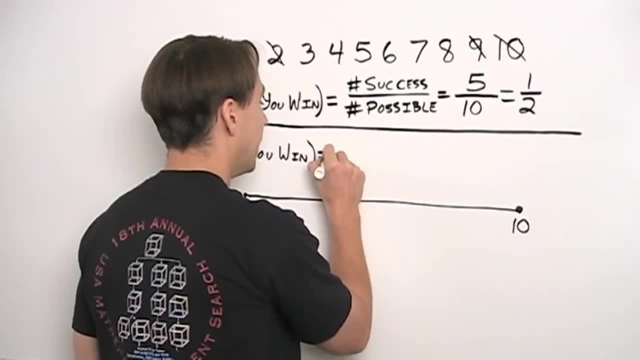 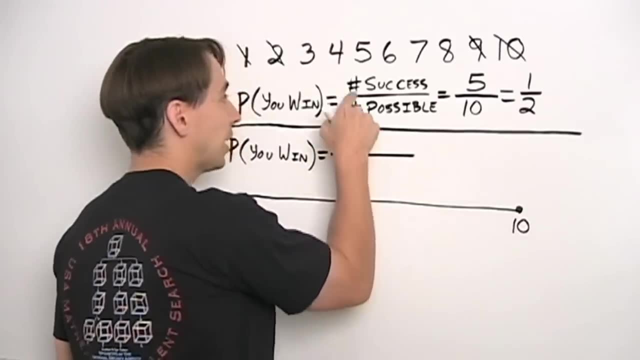 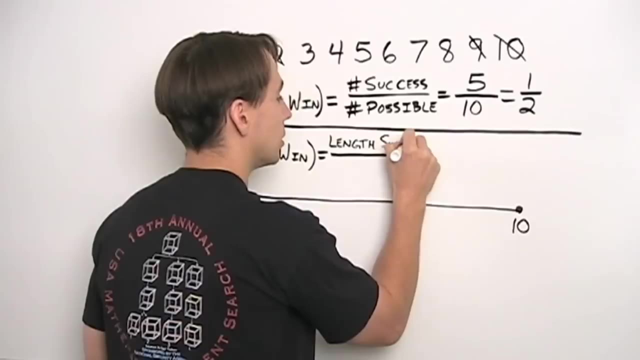 The length of this segment from 1 to 10 is 9.. And that gives us an idea of how to find the probability. Instead of counting the number of successes, we're going to count the length of the successful region, And we're going to divide by the length of the possible region. 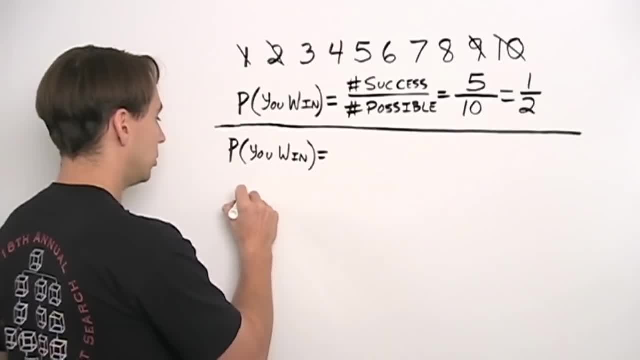 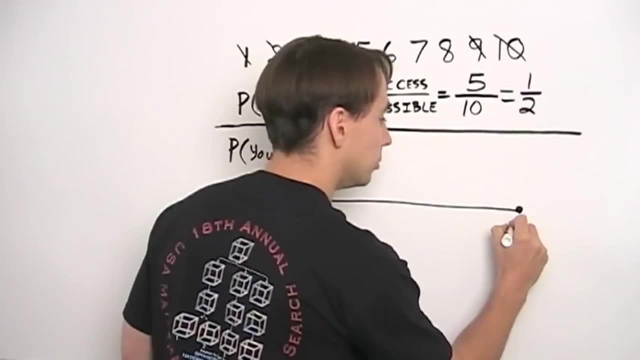 Let's go ahead and look at that. We'll go ahead and draw a number line. Here's our number line And our number line goes from 1 to 10.. Because I can choose any number on the number line from 1 to 10.. 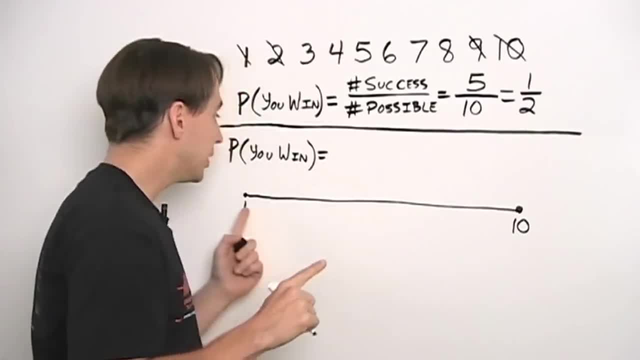 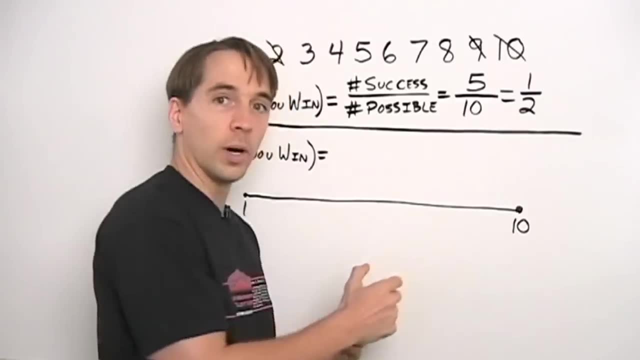 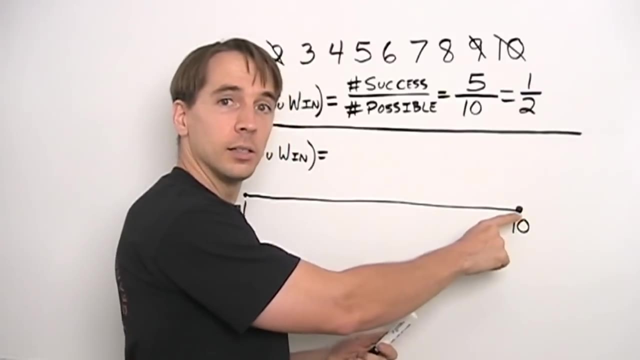 And aha, now we see a way to measure our possible region. There are tools to measure these continuous quantities. Geometry has them, And one of those tools is length. I can pick any number from 1 to 10.. And the length of this region is 9.. 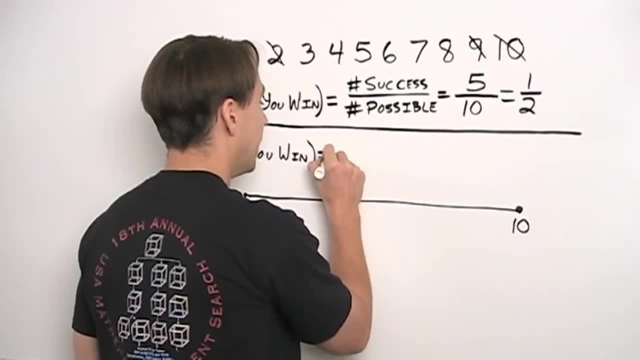 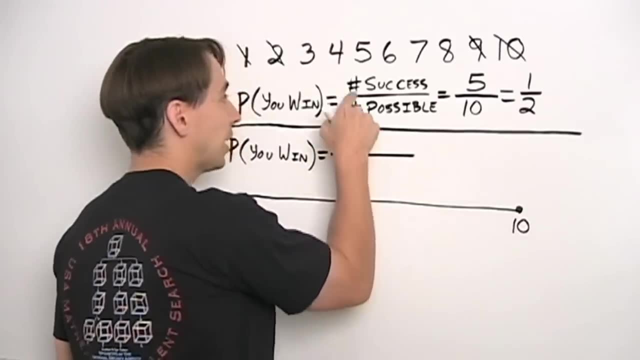 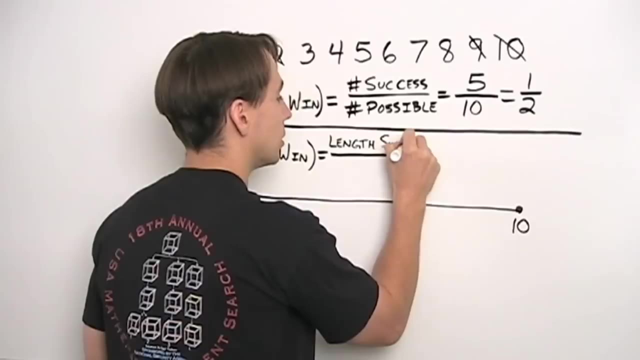 The length of this segment from 1 to 10 is 9.. And that gives us an idea of how to find the probability. Instead of counting the number of successes, we're going to count the length of the successful region, And we're going to divide by the length of the possible region. 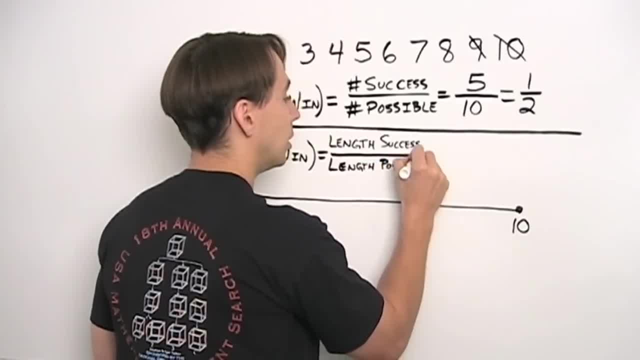 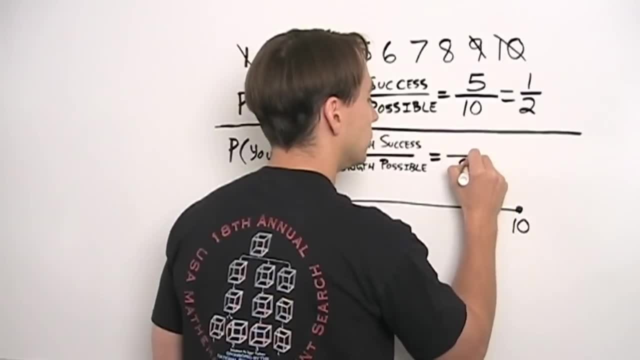 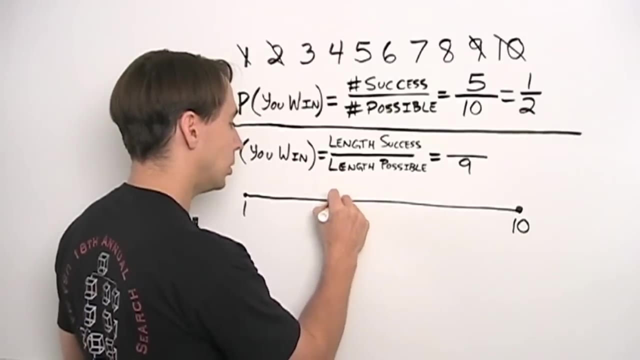 And we can see right here already we've got our possible region. It's 9 long. What's the length of our successful region? Well, say, you picked a number right here, You're going to win $1,000. if my number is within 2 of that. 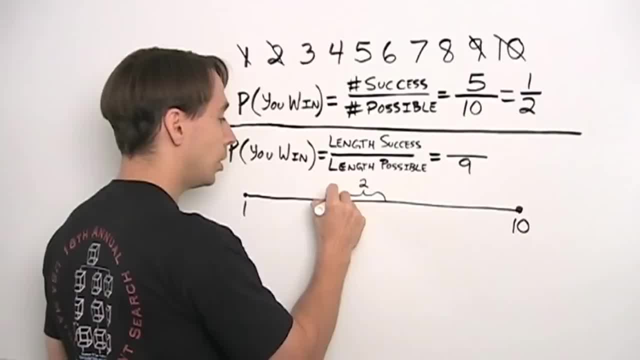 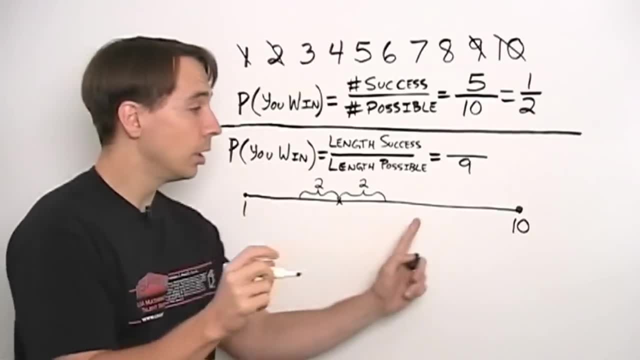 So that's within 2 above or within 2 below And, as we discussed up here, you're not going to pick a number any lower than 3 or a number any higher than 8.. You're going to pick 3 or 8 and cover even more area. 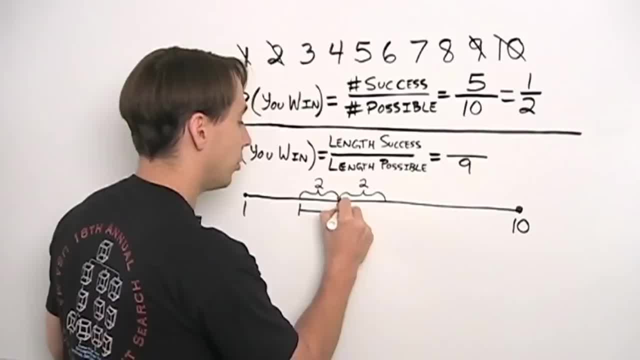 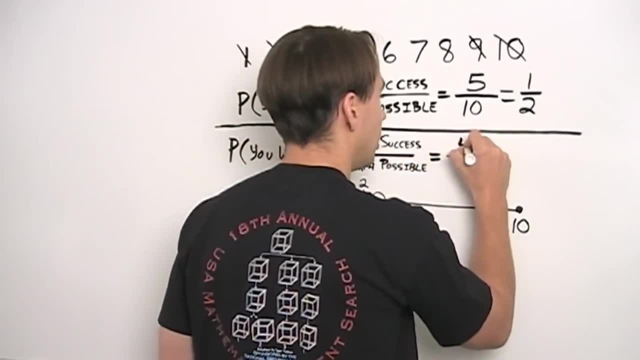 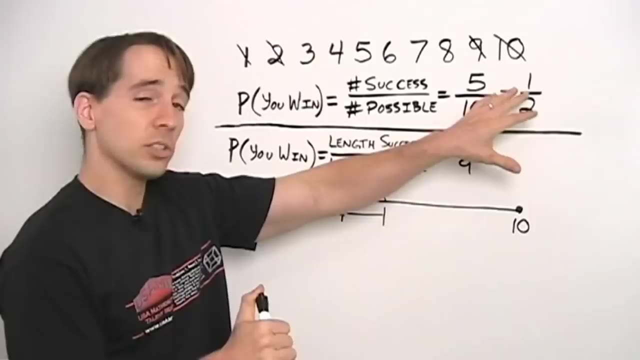 So the total length of the region where you win is 4.. So the length of the successful region is 4.. The length of the possible region is 9.. The probability that you win $1,000 is 4- nines. It's still pretty good. 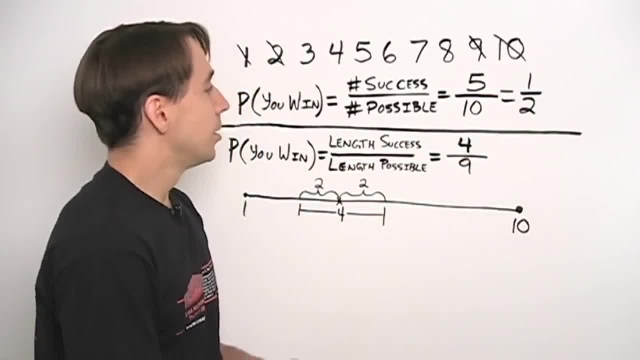 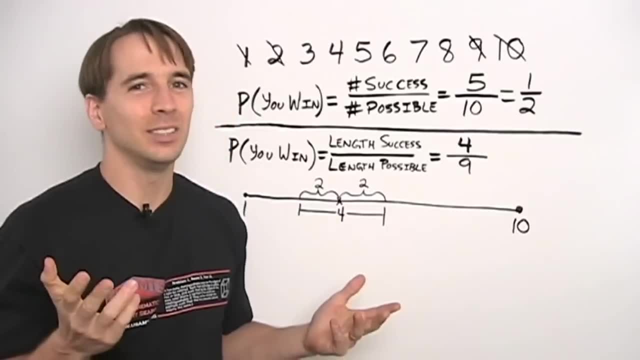 It's not as good as a half. I'm a nice guy, but I'm not that nice. It's still a pretty good chance. Now let's hear your number. What was that? Sorry, you missed. You missed by 2.4..